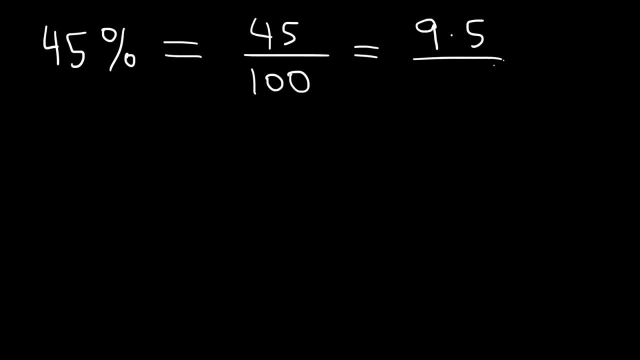 It turns out that 45 is 9 times 5. And 100 is 20 times 5.. You can find the numbers 9 and 20 by dividing 45 by 5 and 100 divided by 5. You'll get the 9 and 20.. 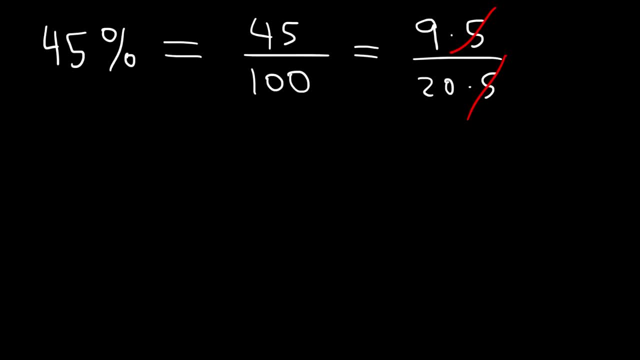 But we can cancel a 5. And that's as far as we can go. So 45% is equivalent to 9 over 20.. 9 over 20 as a reduced fraction And this is the answer for that example. 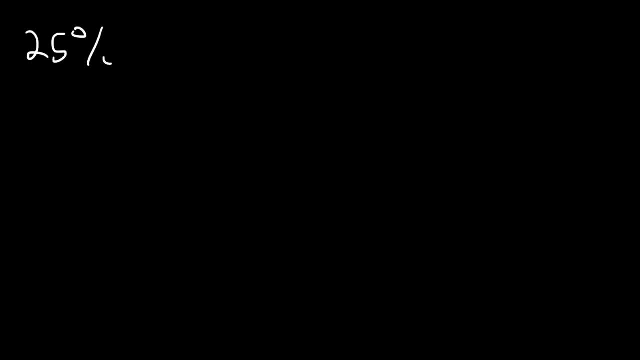 Go ahead and try these two: Convert 25% into a reduced fraction And do the same for 36%. So let's start by writing this as 25 divided by 100.. 25 is 5 times 5.. 100 is 20 times 5.. 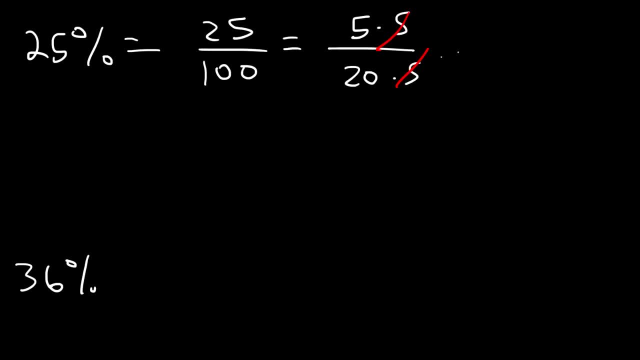 So we can cancel a 5. And we can reduce the fraction. So we can cancel a 5. And we can reduce it further. So right now we have 5 over 20.. It turns out that 20 is 5 times 4.. 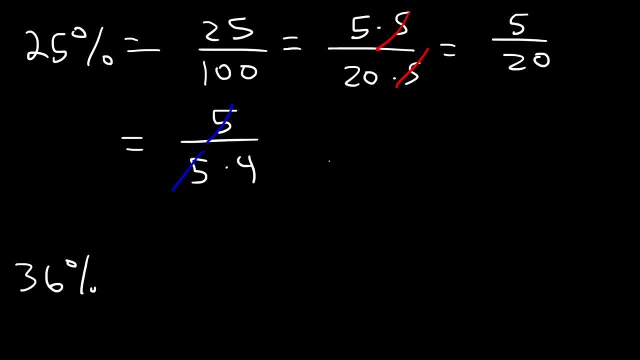 So we can cancel a 5 as well. 5 divided by 5 is 1.. So when you get rid of the 5 on top, replace it with a 1.. Therefore, 25% is equivalent to 1. fourth, as a simplified fraction: 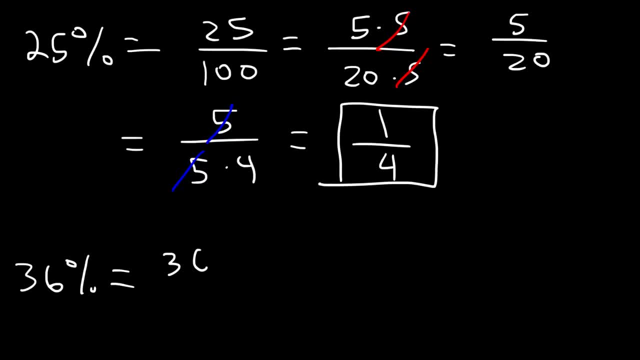 Now let's do the same thing with 36%. Let's write it as 36 over 100.. Now 36 is 9 times 4.. 100 is 25 times 4.. So we can cancel a 4.. 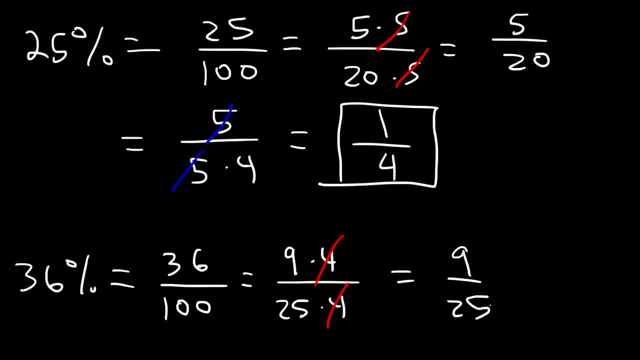 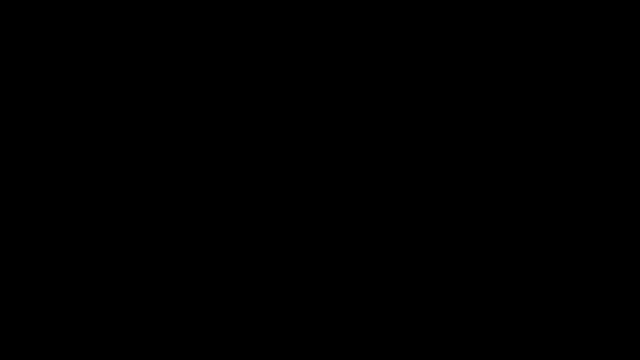 And we're left with just 9 over 25.. And that's the answer. So 36% is equivalent to this fraction. So now you know a simplified way of converting percentages into fractions. Now, sometimes you may have a percentage that exceeds 100.. 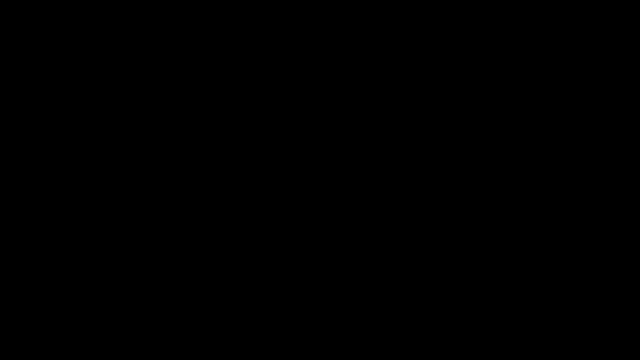 And sometimes you may have a percentage that exceeds 100.. And when you have those, you can convert your answer to an improper fraction. Or sometimes you may need to convert it to a mixed number. So here's an example: Convert 140% into a fraction. 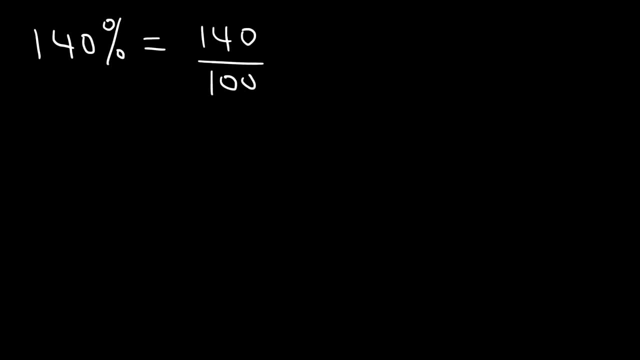 So 140% is basically 140 divided by 100.. Now the first thing we need to do is reduce the fraction. 140 is 14 times 10.. 100 is 10 times 10.. So we can cancel a 10.. 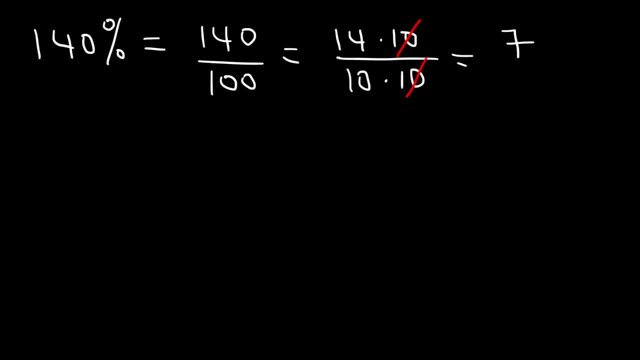 But we can reduce it further. 14 is 7 times 2. And 10 is 5 times 2.. So we can get rid of a 2. So as an improper fraction, 140% is 7 divided by 5.. 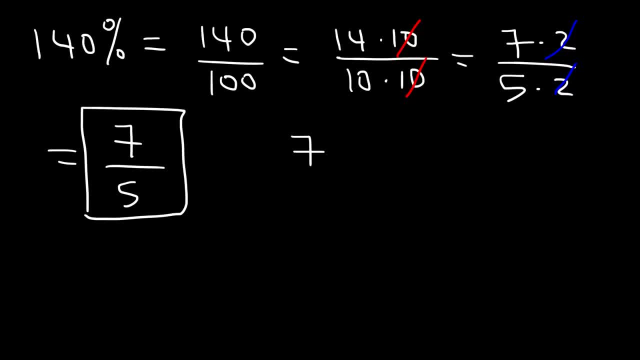 Now we can convert this into a mixed number. 7 is basically 5 plus 2.. Now let's keep the denominator the same: 5 divided by 5 is 1.. So we have 1 plus 2. fifths, 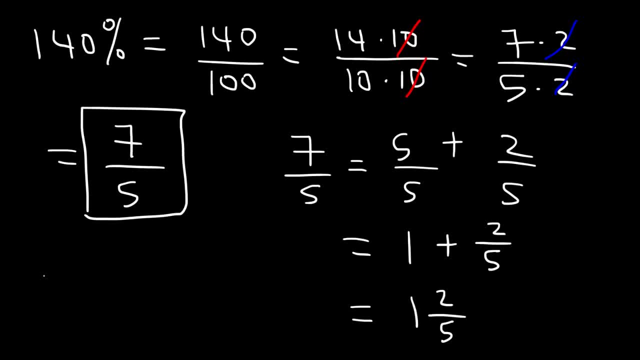 So as a mixed number, it's 1 and 2 fifths Now. granted, you could use long division to convert an improper fraction to a mixed number, But sometimes you may need to report your answer as an improper fraction, Other times you may need to report it as a mixed number. 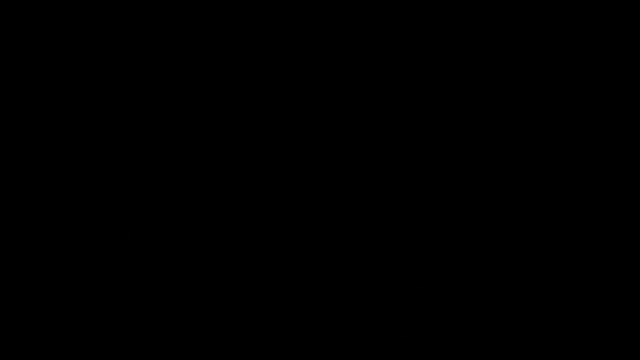 So we're going to do it both ways. Now go ahead and try this one for practice. Convert 280% into an improper fraction And a mixed number, So let's divide it by 100.. 280 is 28 times 10.. 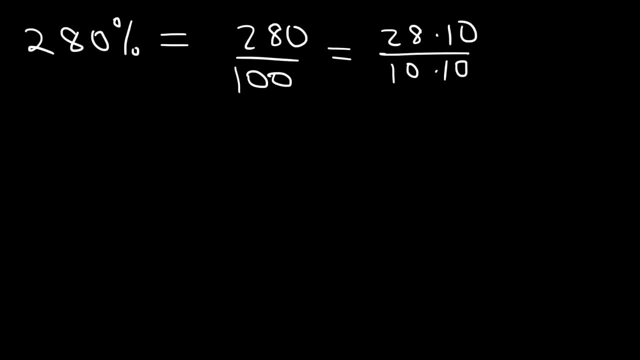 And we know 100 is 10 times 10.. 28 is 14 times 2. And 10 is 5 times 2.. So therefore our answer, as a reduced improper fraction, is 14 over 5.. Now let's convert that into a mixed number using long division. 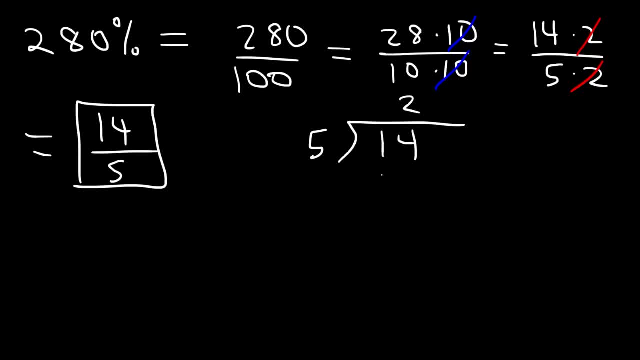 5 goes into 14 two times. 5 times 2 is 10.. And 14 minus 10 is 4.. So since 5 goes into 14 two times, we're going to have a 2 as a whole number. 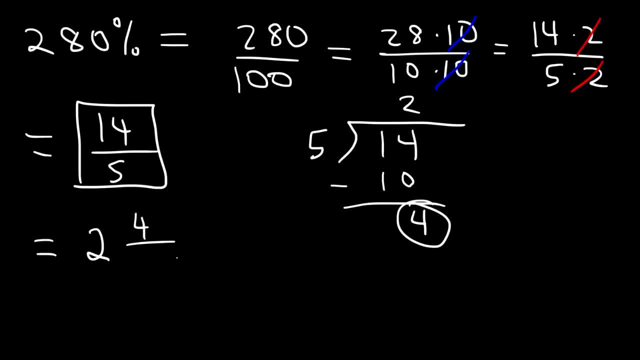 And the 4, the remainder will be the numerator of the mixed number And 5 will remain the denominator. So 14 over 5 is basically 2 and 4 fifths as a mixed number, Which is the denominator. 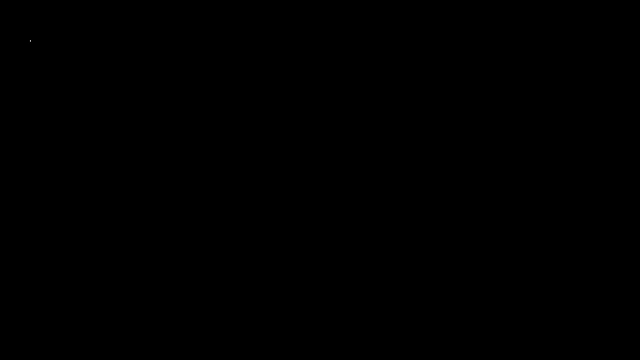 So that equates to 280 percent. Here's another example: 335 percent. Let's convert that into a fraction. So take a minute, pause the video and try that. So let's divide it by 100 first. 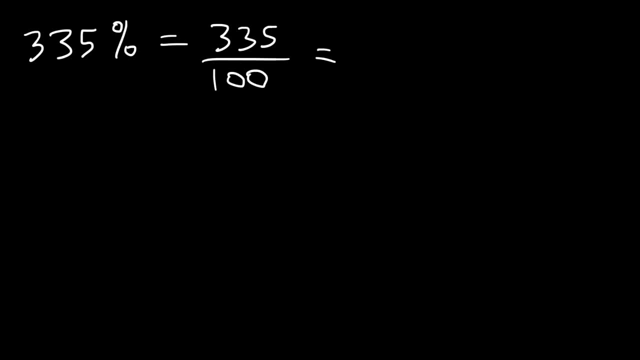 Now, 335 is divisible by 5.. If you divide it by 5, you're going to get 67. So we can write it as 67. 67 times 5.. And 100 is 20 times 5.. 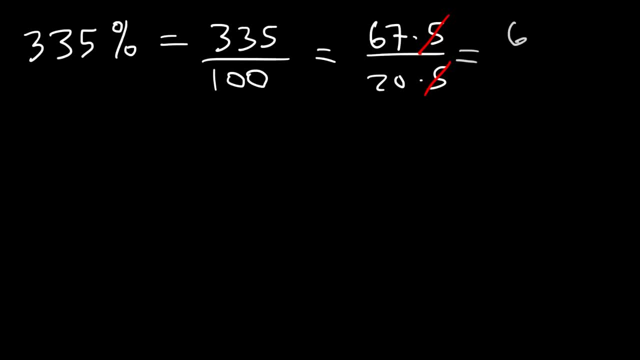 Now we can't really break down 67 into anything. 2 doesn't go into it, and 3 doesn't go into it either, So we can't break it down into anything useful. So therefore we're going to leave our answer as an improper fraction, just like that. 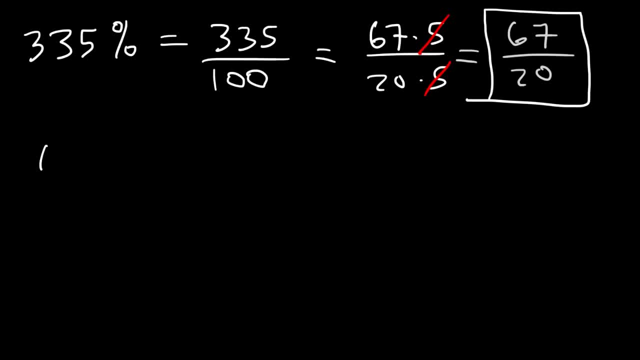 Now let's convert this into a mixed number, So I'm going to break it down into 67.. 60 and 7.. Because 20 goes into 60. nicely, 60 divided by 20 is 3.. So it's 3 plus 7 over 20.. 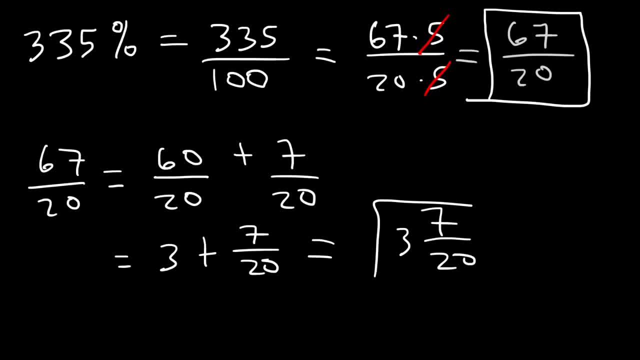 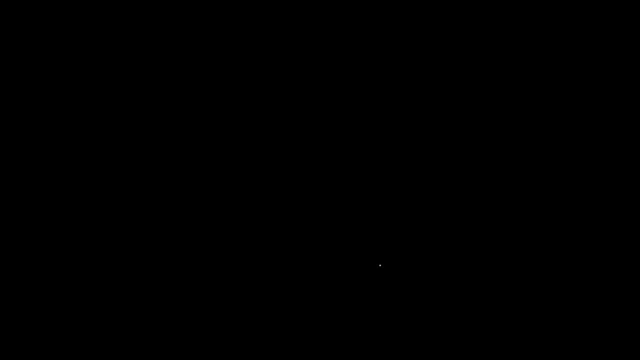 And here's the answer- as a mixed fraction, 3 and 720.. And so that's it. That's all you've got to do Now. other times you may need to convert a percentage into a fraction where the percentage is less than 1.. 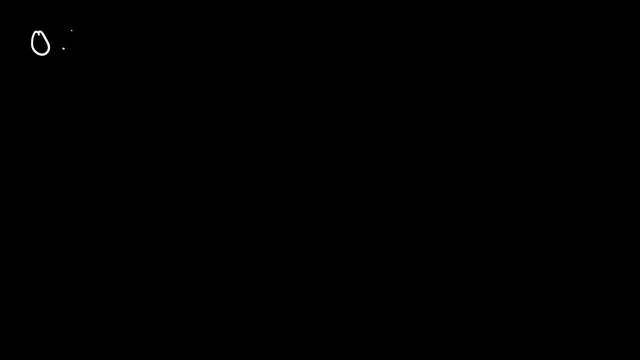 It's a decimal value, So it's like a very small number. Let's convert 0.15% into a fraction, So let's start with the same technique. Let's divide it by 100.. Now, 0.15 is a very small number. 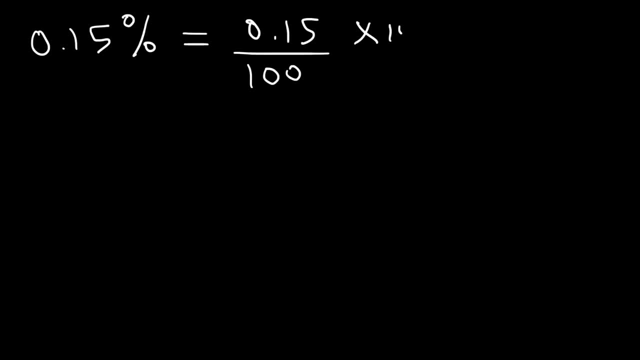 So let's make it larger by multiplying the top and the bottom by 100.. Notice that 0.15 goes to the 100th place. So to get rid of the decimal, you want to multiply it by 100.. 0.15 times 100 is 15.. 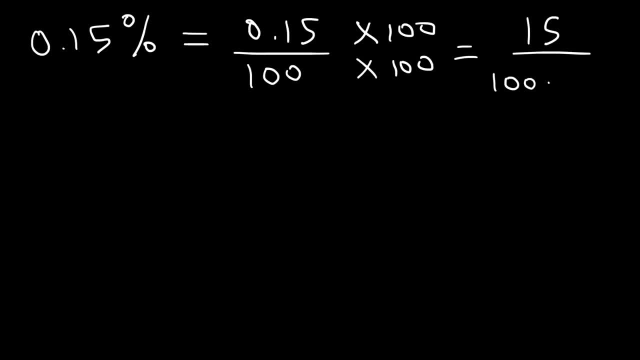 100 times 100 is 10,000. But I'm just going to leave it there. I'm going to leave it as 100 times 100 for now. Now, 15 is 5 times 3.. And one of the 100 values. I'm going to write it as 20 times 5.. 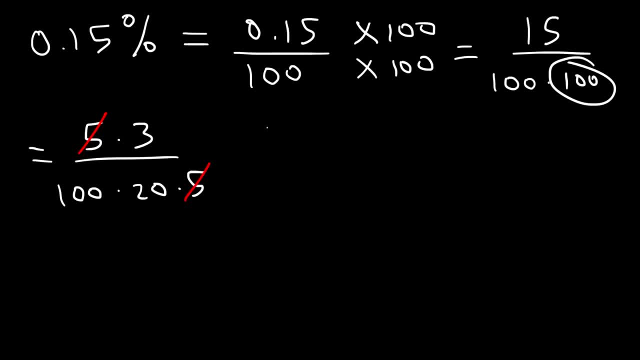 So I can get rid of a 5.. So I'm left over with a 3 on top On the bottom, 100 times 20.. If you have $120 bills, you have $2,000.. So our answer is going to be 3 over 2,000. 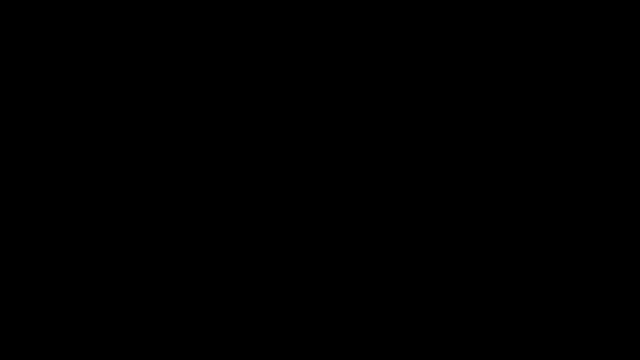 That equates to 0.15%. Here's another example. Convert 0.025% into a fraction. So first let's write it over 100.. So this is 0.025 divided by 100.. Now, in order to turn 0.025 into a whole number, 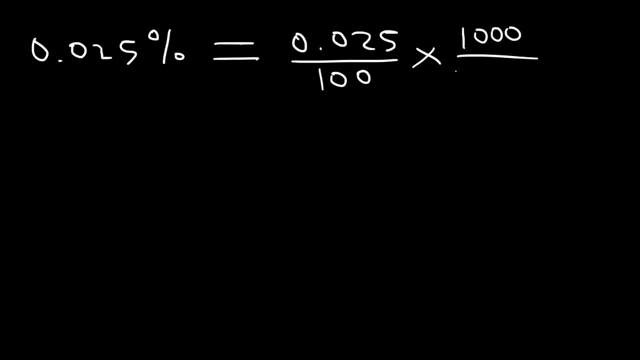 we need to multiply the top and the bottom by 1,000. Because the last number is in the 1,000th place. 0.025 times 1,000 is simply. You just got to move the decimal three units to the right. 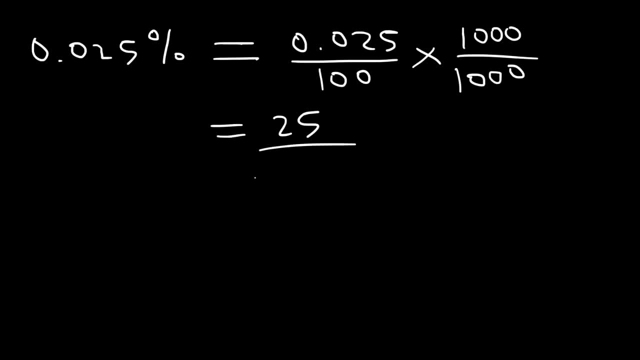 So that's going to be 25.. And on the bottom I'm just going to rewrite: 100 times 1,000.. Now, 100, we can write that as 25 times 4.. We're not going to do anything with 1,000 for now. 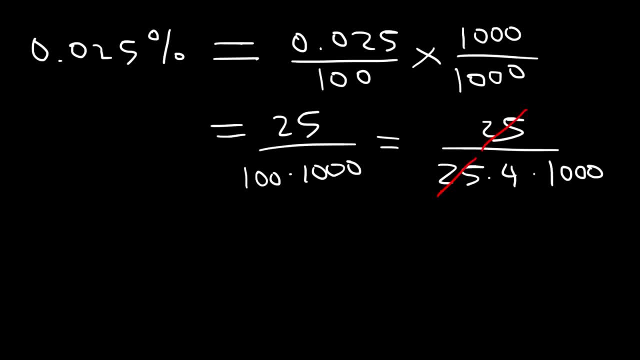 But notice that we can cancel the 25.. Now, 1,000 times 4 is 4.5. So that's going to be 25.. So the final answer is 1 divided by 4,000.. So that equates to that number that we had in the beginning. 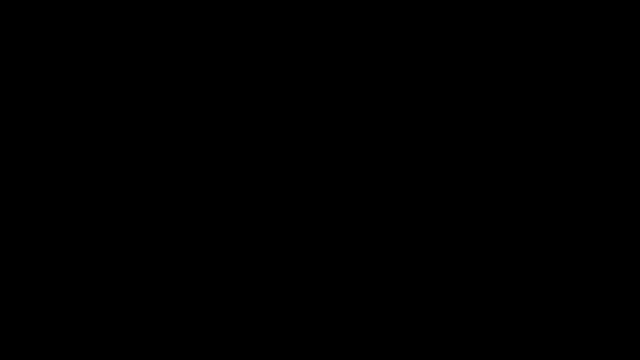 Now, sometimes you may have a percentage presented to you as a mixed number, For example, 32 and 1 third percent. How do you convert that into a fraction? Well, let's start with the same process. Let's take this number and divide it by 100.. 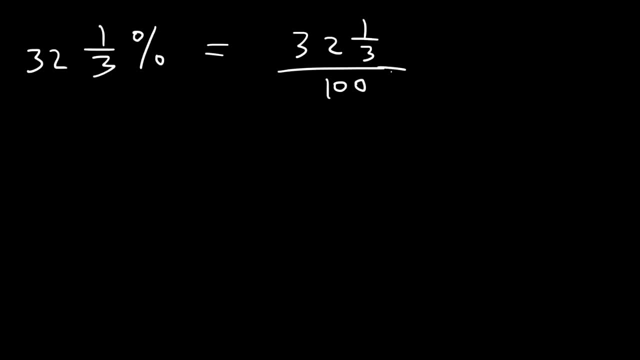 Now what you want to do is you want to convert the mixed number into an improper fraction. To do that, multiply 32 by 3, which is 96, and then add 1.. That's 97.. So 32 and 1 third is going to be 97 divided by 3.. 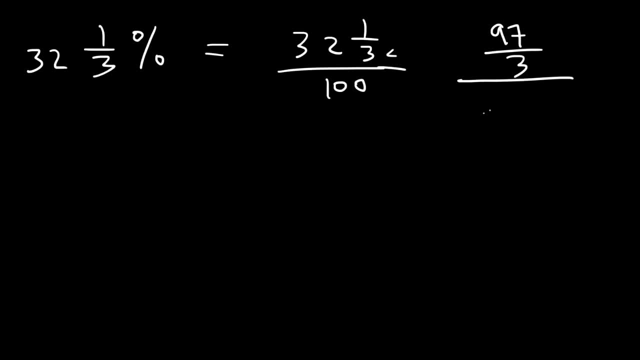 The denominator stays the same. Now 100, I'm going to write that as a fraction. 100 is equal to 100 over 1.. So we have this fraction divided by this fraction, Which we can write that as a fraction. 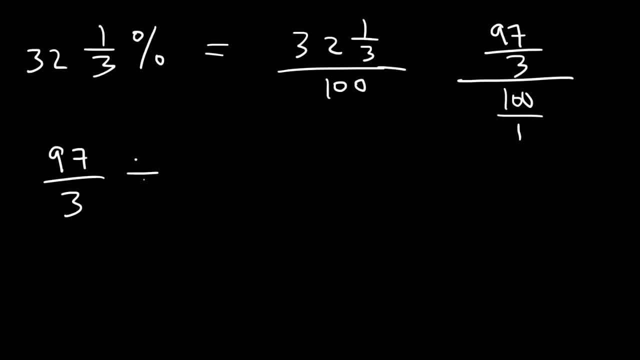 So we can write that expression as 97 over 3, divided by 100 over 1.. Now, using the keep-change-flip principle, we can keep the first fraction, the same change division to multiplication, and flip the second fraction.